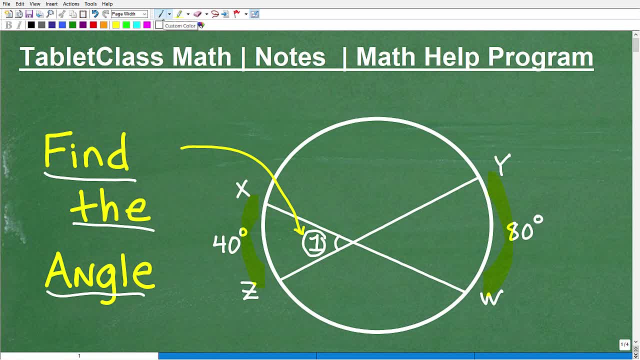 And the angle here is 80 degrees. So this is a very typical high school level geometry type of problem And typically you know you don't study this stuff in like algebra courses or like pre-calculus or whatnot. This is pretty much all contained, for the most part, in like a high school level geometry course. But you need to know this Matter of fact. I just got done doing a video on the SAT and the ACT math section. So if you're in high school you're going to need to know this. 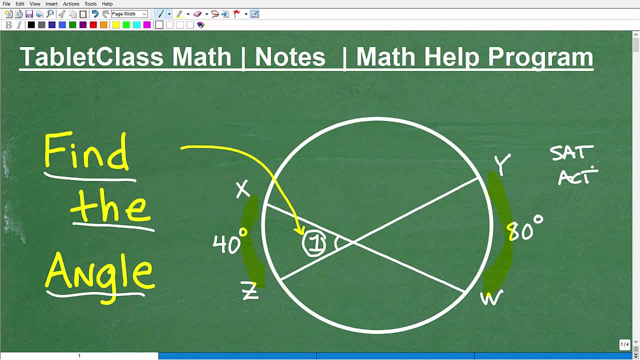 If you're in high school level geometry, you know it's a good chance. you might be thinking about going to college, which means you might be taking one of these exams. Now, in order to solve this problem, we need to know a formula. Now you might be saying, well, where am I going with this? Well, let me just make my point here real quick. So you need to know a formula to solve this particular problem. So if you forget the formula, well you know that's going to be an issue if you decide to take the ACT because there's no formula sheet. 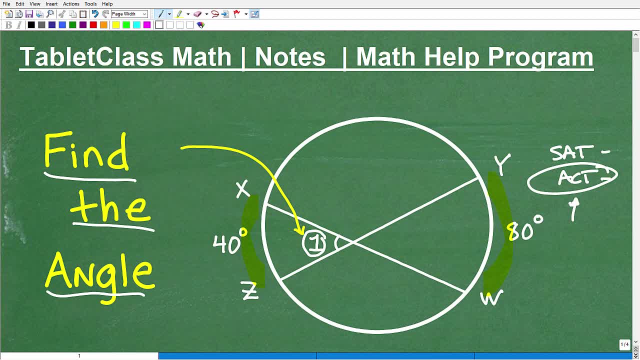 So you have to kind of remember this stuff, And in mathematics it's just the way it is. There's a lot of formulas and theorems and things that you do have to remember. You can't possibly remember everything. That's why we take notes, And I'm going to get to that in a second. But on the SAT there is a reference sheet that you can use. But even on that reference sheet you may not have the formula you need for this particular problem. So the bottom line is: you know, if you feel overwhelmed with all the formulas that you're learning in math, you're going to have to remember everything. 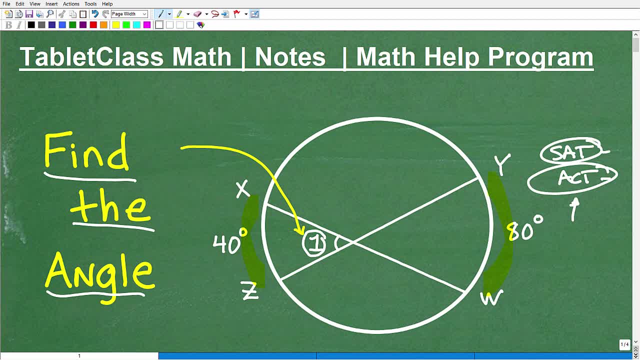 In mathematics or, you know, in school. it is what it is And that's why it's critical to take excellent notes and really work on your retention, which I'm going to get into in a second. But this formula here is not too difficult And we're going to solve this problem. It's a pretty easy problem to solve. But again, if you don't know the formula, you know, if you don't know what to do, then you know you're just kind of guessing and we want to avoid that at all costs. But before we get into this problem, let me quickly introduce myself. My name is John. I'm the founder of the 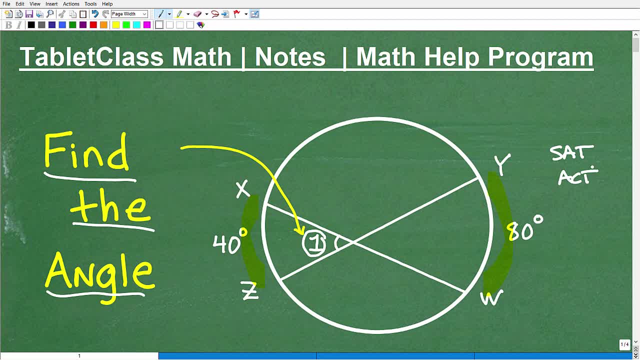 If you're in high school level geometry, you know it's a good chance. you might be thinking about going to college, which means you might be taking one of these exams. Now, in order to solve this problem, we need to know a formula. Now you might be saying, well, where am I going with this? Well, let me just make my point here real quick. So you need to know a formula to solve this particular problem. So if you forget the formula, well you know that's going to be an issue if you decide to take the ACT because there's no formula sheet. 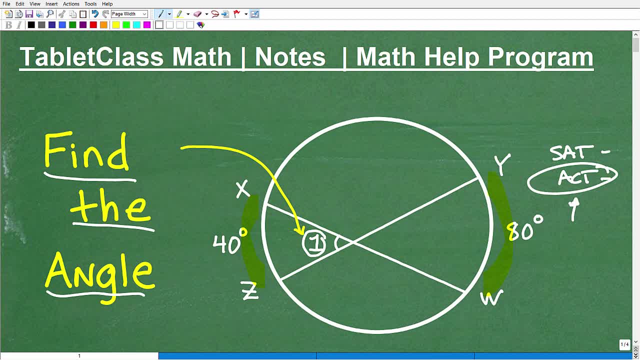 There's no real formula sheet, There's no reference sheet. So you have to kind of remember this stuff. And in mathematics it's just the way it is. There's a lot of formulas and theorems and things that you do have to remember. You can't possibly remember everything. That's why we take notes- And I'm going to get to that in a second. But on the SAT there is a reference sheet that you can use. But even on that reference sheet you may not have the formula you need for this particular problem. So the bottom line is: you know, if you feel overwhelmed with all the formulas that you're learning in mathematics, you're going to have to remember everything. 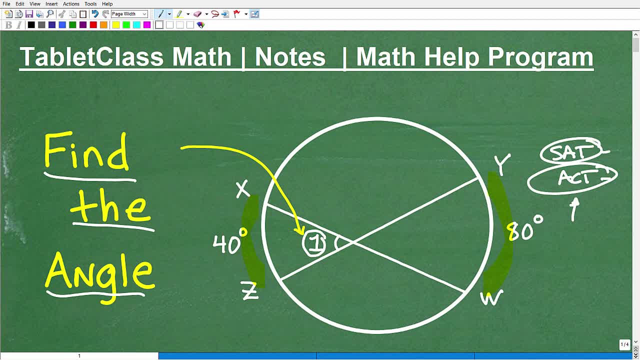 So if you're learning mathematics or you know in school, it is what it is And that's why it's critical to take excellent notes and really work on your retention, which I'm going to get into in a second. But this formula here is not too difficult And we're going to solve this problem. It's a pretty easy problem to solve. But, again, if you don't know the formula, you know, if you don't know what to do, then you know, you're just kind of guessing and we want to avoid that at all costs. But before we get into this problem, let me quickly introduce myself. My name is John. I'm the founder of the SAT. 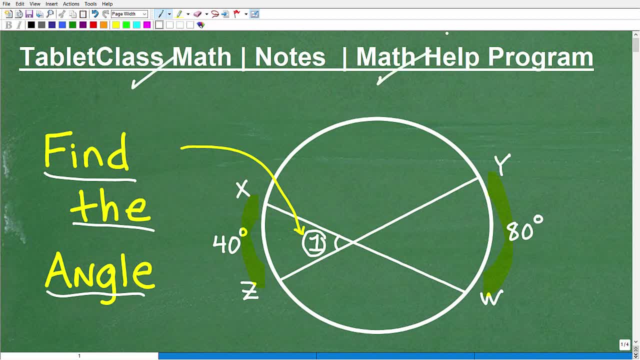 I'm also a middle and high school math teacher And over several years I've constructed what I like to believe is one of the best online math help programs there is. Of course, I'll let you be the judge of that. You can check out my math help program by following the link in the description of this video. But basically I have all the main math courses, like pre-algebra, algebra one, geometry- So if you take a geometry, it could definitely help you out. I also have algebra two. I'm going to be launching pre-calculus here shortly, But I also have a lot of tests in the area of math. 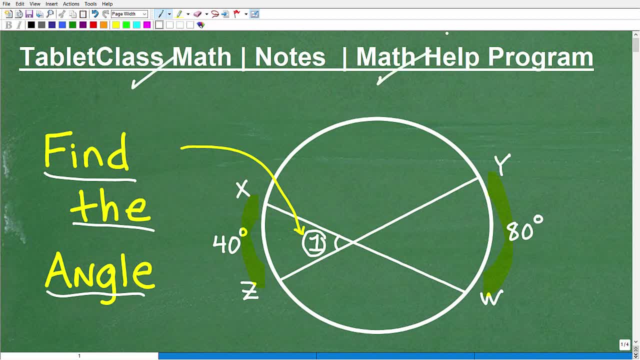 Tablet Class Math. I'm also a middle and high school math teacher And over several years I've constructed what I like to believe is one of the best online math help programs there is. Of course, I'll let you be the judge of that. You can check out my math help program by following the link in the description of this video. But basically I have all the main math courses like pre-algebra, algebra one, geometry- So if you take a geometry, I could definitely help you out. I also have algebra two. I'm going to be launching pre-calculus here shortly- But I also have a lot of tests in the area of 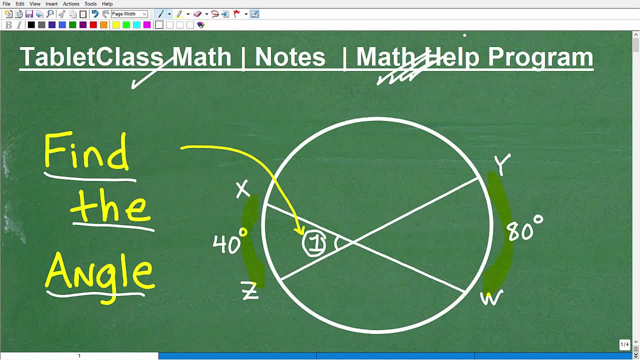 test preparation. There's a lot of courses in the area of test preparations, like the GED. So if you're taking the GED or the SAT, ACT, GRE, GMAT, maybe a teacher certification exam, CLEP exam, Alex Accuplacer, nursing entrance exam- all those exams I mentioned have a lot of mathematics on those on the exams And if you don't get to the math sections you don't get to the exam. So if you're preparing for one of these exams, just go to my site and check out my full course. 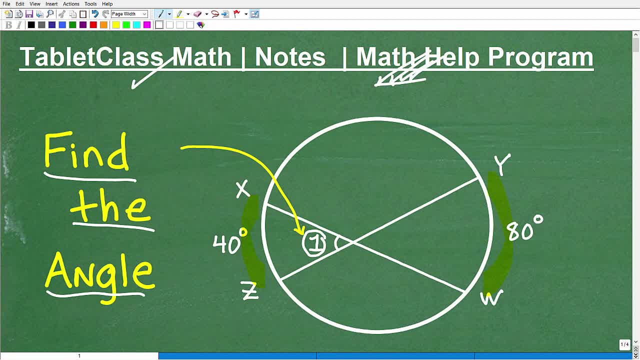 I should have what you need If I don't, drop me a line and I'll help you out the best I can. I also do a lot with independent learners, like homeschoolers. I have a great homeschool learning system, And then, obviously, I help those of you that are struggling in your current math course. So if you're having a tough time in geometry, you may want to check out my full geometry course. It will definitely help you out. Now, one of the things I can't do for you that you must do for yourself, that is the following: You got to take great math notes. I've been teaching math for decades And it's apparent to me that those students who 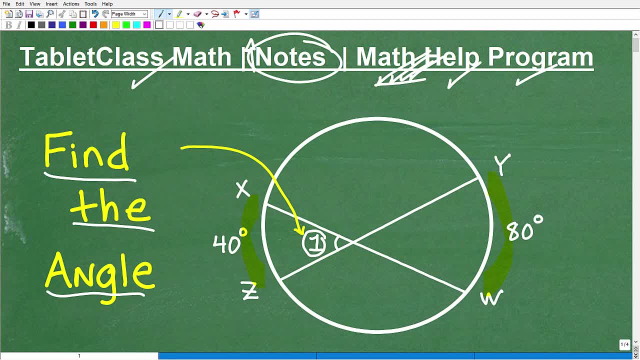 put the work in and have excellent math notes, almost do very well in all their tests and and even on other tests like the SAT and ACT. And then the reverse is true, Those students who just don't bother take notes or inconsistent inner note taking, or like to talk to their best buddies or look at their cell phone during math class. well, you get the picture. you know they end up having a difficult time. And the thing is this: like this particular problem, we need a formula. If you weren't paying attention, 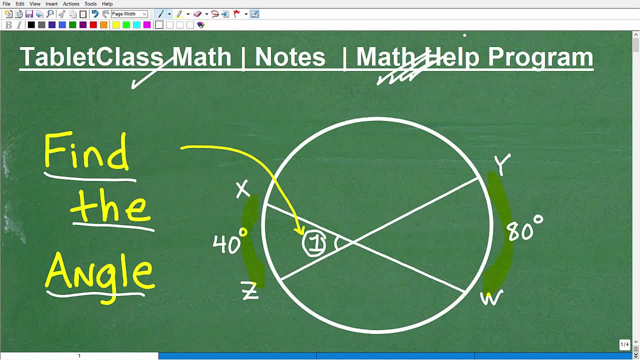 Test preparation. There's a lot of courses in the area of test preparations, like the GED. So if you're taking the GED or the SAT, ACT, GRE, GMAT, maybe a teacher certification exam, CLEP exam, Alex Accuplacer, nursing entrance exam- All those exams I mentioned- have a lot of mathematics on those on the exams And if you don't get to the math sections you don't get to the exam. So if you're preparing for one of these exams, just go to my site and check out my full course. 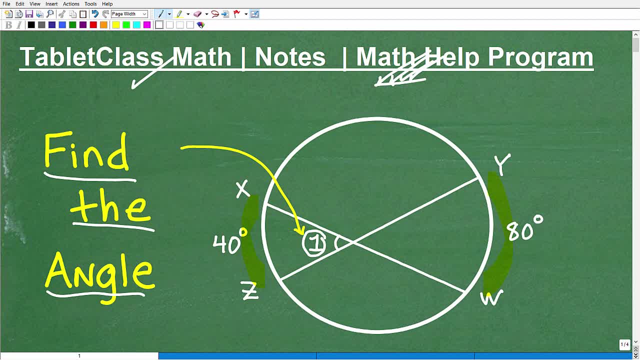 Catalog. I should have what you need. If I don't, drop me a line and I'll help you out the best. I can Also do a lot with independent learners like homeschoolers. I have a great homeschool learning system, And then, obviously, I help those of you that are struggling in your current math course. So if you're having a tough time in geometry, you may want to check out my full geometry course. It will definitely help you out. Now, one of the things I can't do for you that you must do for yourself, That is the following: You got to take great math notes. I've been teaching math for decades And it's apparent to me that those students who 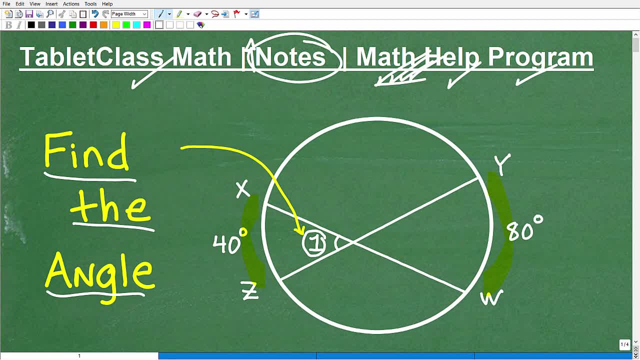 put the work in and have excellent math notes, almost do very well And all their tests and and even on other tests like the SAT and ACT. And then the reverse is true, Those students who just don't bother take notes or inconsistent inner note taking, or like to talk to their best buddies or look at their cell phone during math class. well, you get the picture. you know they end up having a difficult time. And the thing is this: like this particular problem, we need a formula. If you weren't paying attention, 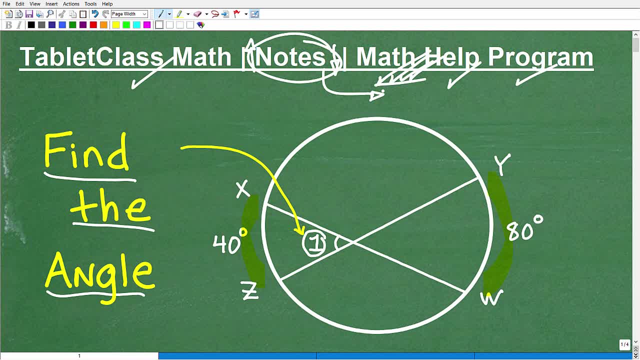 and you didn't write that formula down in your notes, how would you be able to do these problems in the homework right? So, again, the whole key to learning anything is focus right, And there's no better activity than note taking to keep you focused. Just trust me on this one: Really work on your notes. As you improve your notes, everything else will be improved. But as you're improving, I actually offer detailed, comprehensive math notes to include pre-algebra, algebra one, geometry, algebra two and trigonometry. You can find the links to: 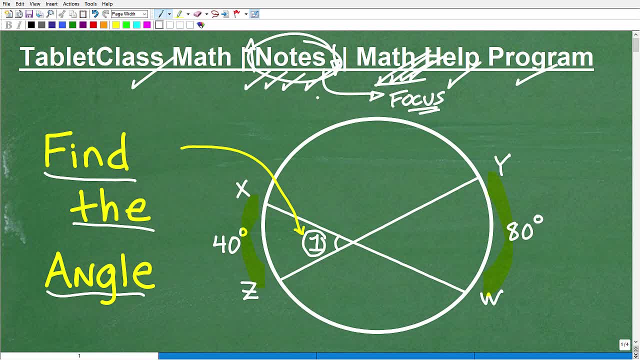 those notes in the description of this video. Now, of course, if you know how to solve this problem, if you think you know how to do it without guessing, I would certainly encourage you to pause the video and go ahead and do so. But we're going to get into the solution now. 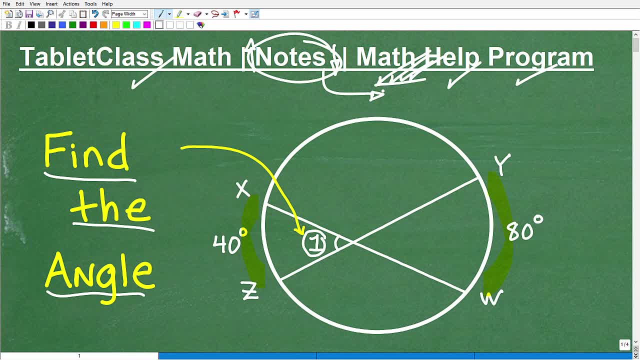 and you didn't write that formula down in your notes, how would you be able to do these problems in the homework right? So, again, the whole key to learning anything is focus right, And there's no better activity than note taking to keep you focused. Just trust me on this one: really work on your notes. As you improve your notes, everything else will be improved. But as you're improving, I actually offer detailed, comprehensive math notes to include pre-algebra, algebra one, geometry, algebra two and trigonometry. You can find the links to 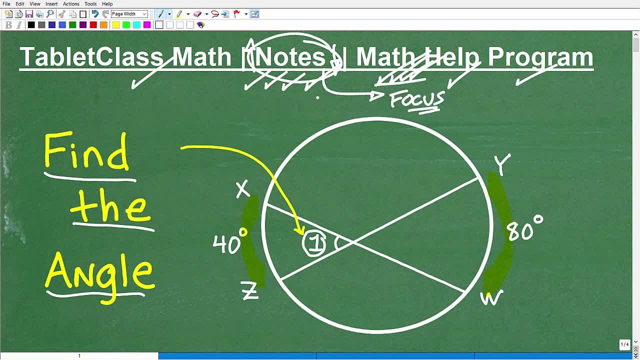 those notes in the description of this video. Now, of course, if you know how to solve this problem, if you think you know how to do it without guessing, I would certainly encourage you to pause the video and go ahead and do so. But we're going to get into the solution now. 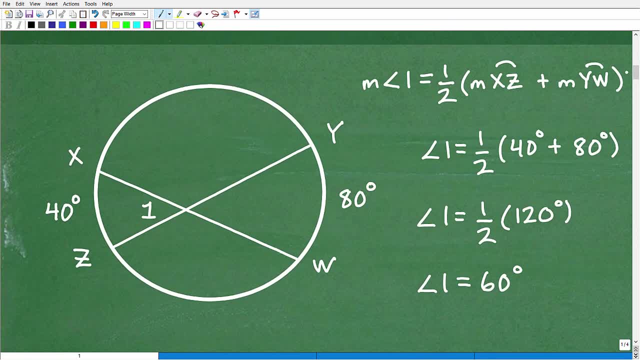 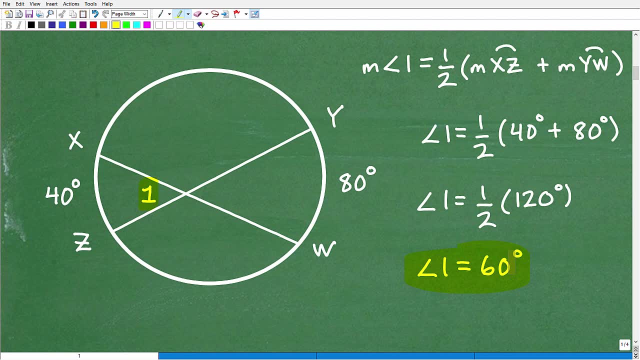 Okay, so here it is Again doesn't require a lot of work, But the answer is: angle one is equal to 60 degrees. Okay, All right, So let's go ahead and take a look at our formula here. So there's a. 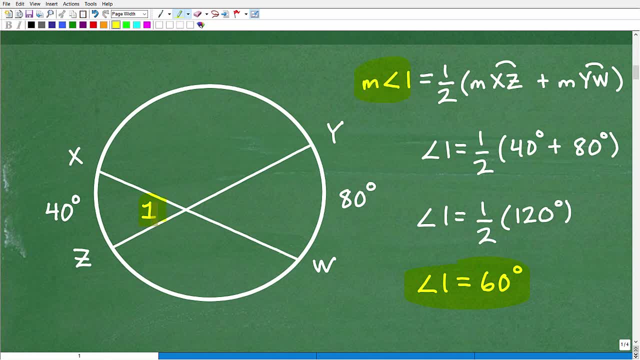 formula in geometry And it states that the measure okay and there's intercepted chords, inscribed chords. there's a whole bunch of stuff going on here that I really don't want to turn this into a complete chapter lesson because this will run into, like you know, three, four or five. 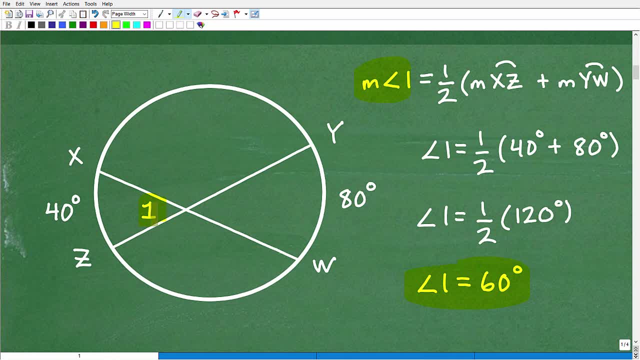 hours to teach you everything about circles. I mean it thoroughly. okay, I could quickly give you the formulas And then you know, but without practicing the formulas that's not going to mean much. So here, when you're trying to find an angle like this where you have two, 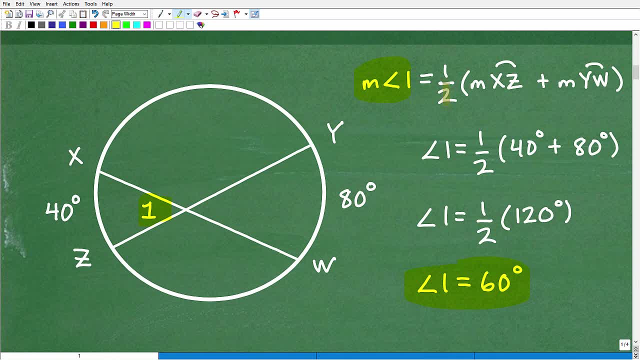 inscribed chords inside of a circle. what we have to do is effectively take the average of the two arcs involved. So we have an arc right here. Okay, And this notation, this little m, means the measure. So we're trying to find the measure of angle one. So if we know the measure, we're going. 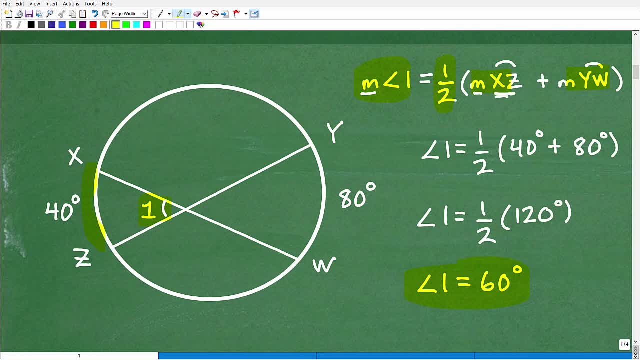 measure of this arc, excuse me right here, XZ. Okay, And we do know the measure of it: It's 40 degrees. And we know the measure of this arc right here, which is YW. Okay, So we add these up and. 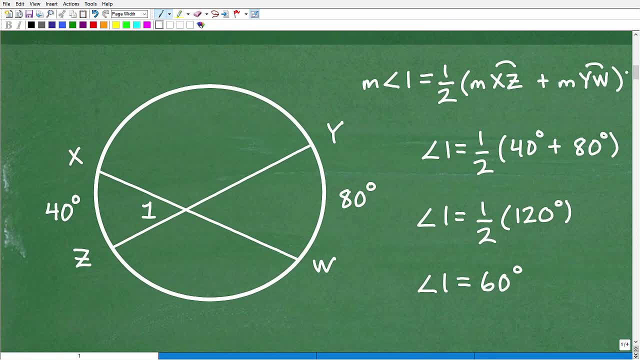 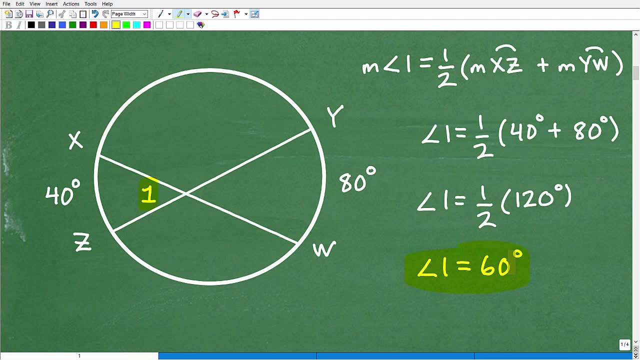 Okay, so here it is Again doesn't require a lot of work, But the answer is: angle one is equal to 60 degrees. Okay, All right, So let's go ahead and take a look at our formula here. So there's a. 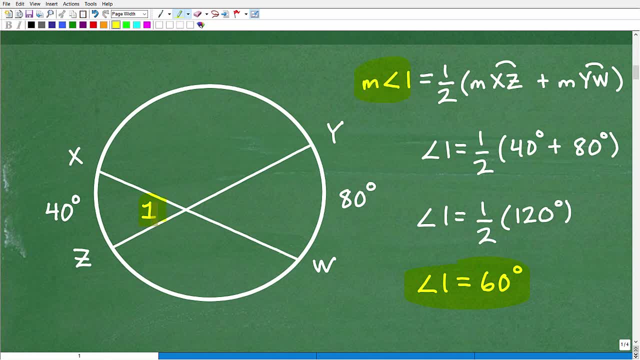 formula in geometry And it states that the measure okay and there's intercepted chords, inscribed chords. there's a whole bunch of stuff going on here that I really don't want to turn this into a complete chapter lesson because this will run into, like you know, three, four or five. 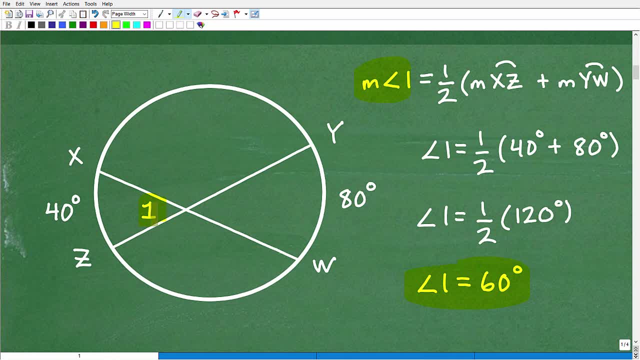 hours to teach you everything about circles. I mean it thoroughly. okay, I could quickly give you the formulas And then you know, but without practicing the formulas that's not going to mean much. So here, when you're trying to find an angle like this where you have two, 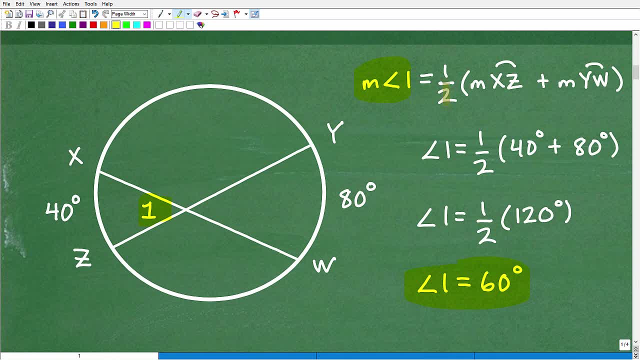 inscribed chords inside of a circle. what we have to do is effectively take the average of the two arcs involved. So we have an arc right here. Okay, And this notation, this little m, means the measure. So we're trying to find the measure of angle one. So if we know the measure of angle one, 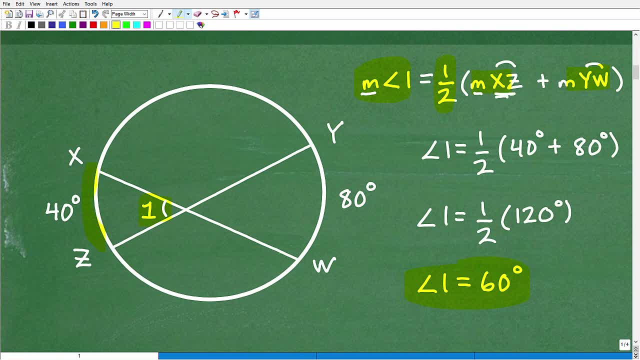 we know the measure of this arc, excuse me right here, XZ. Okay, And we do know the measure of it: It's 40 degrees. And we know the measure of this arc right here, which is YW. Okay, So we add these. 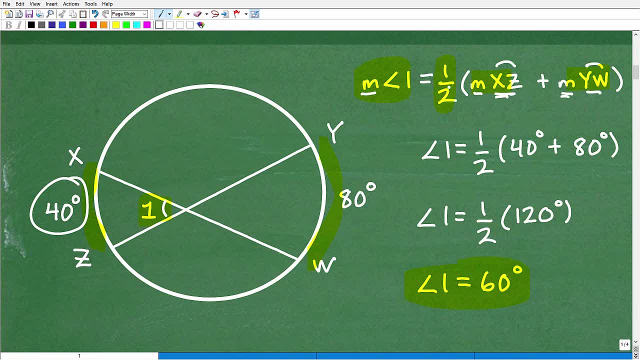 up and just take the average of it, In other words, divide it by two or multiply it by one half. We're going to be able to get this angle right there, Okay, So that's the formula. So we're just going to go ahead and plug in the information. So this is 40 degrees. 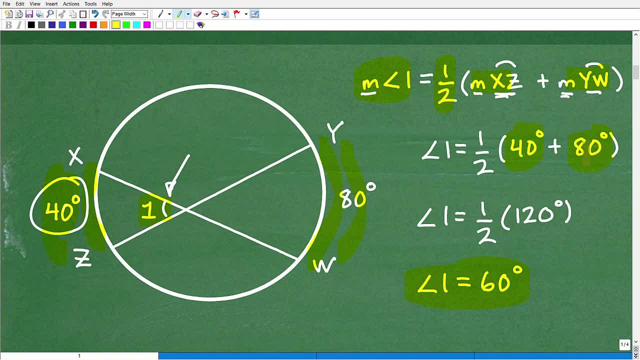 Here, And this is 80 degrees here. So 40 plus 80, that's 120.. We take one half of that, It is 60 degrees, And that is the answer. So again, these problems are not difficult, But if you 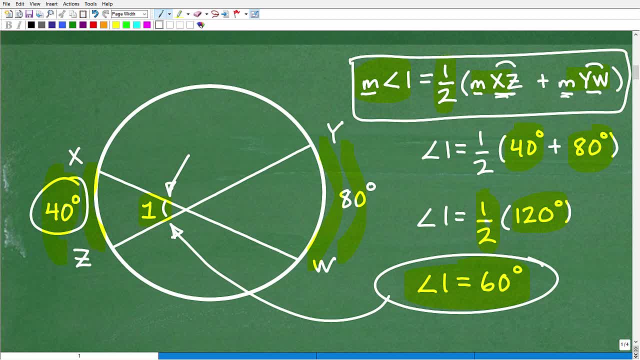 don't know the formula, well then, then you don't know how to do the problem right. So the only way you're going to get good at this is to know the formula and to do a lot of practicing, because there's other formulas involved. Okay, we can be looking for the distances. 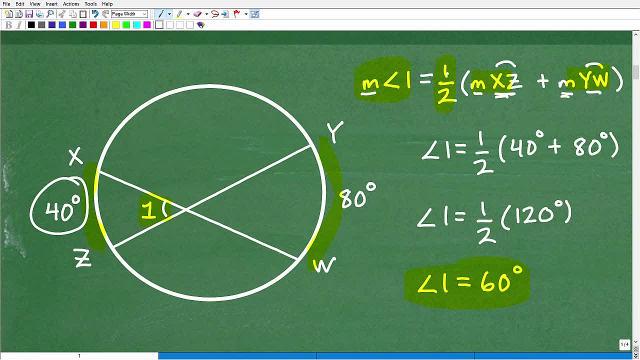 just take the average of it, In other words, divide it by two or multiply it by one half. We're going to be able to get this angle right there, Okay, So that's the formula. So we're just going to go ahead and plug in the information. So this is 40 degrees. 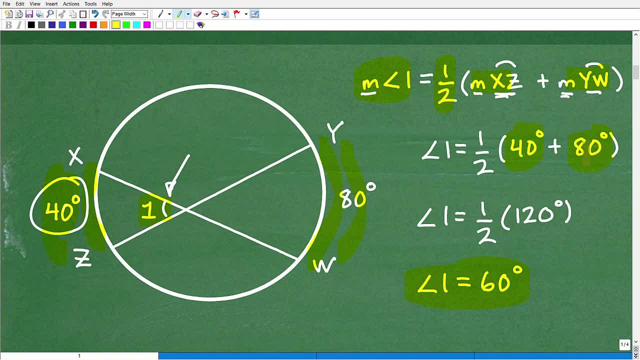 Here, And this is 80 degrees here. So 40 plus 80, that's 120.. We take one half of that, It is 60 degrees, And that is the answer. So again, these problems are not difficult, But if you 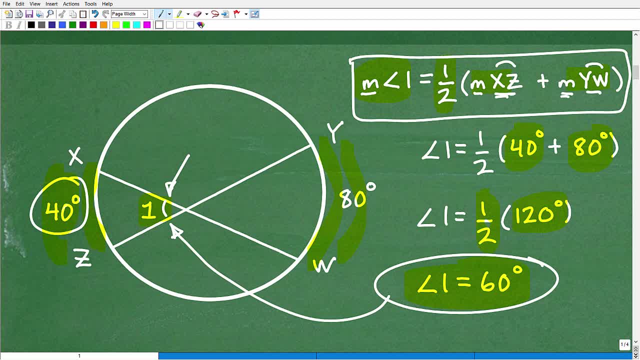 don't know the formula, well then you don't know how to do the problem right. So the only way you're going to get good at this is to know the formula and to do a lot of practicing, because there's other formulas involved. Okay, We can be looking for the distances of these. 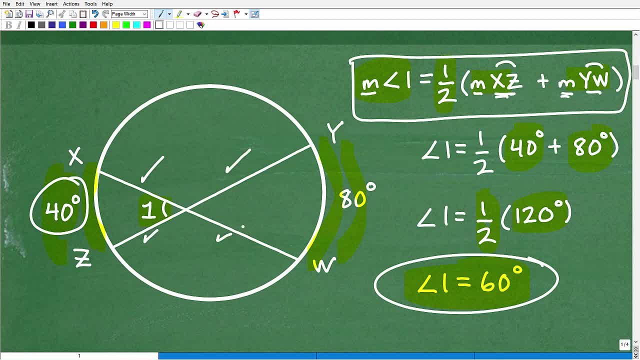 particular lengths here with these cords. There's other things we can be doing. There can be other situations with tangents and things along those lines. So again, it's not just one formula you need to know, especially with respect to circles and geometry, There's quite a bit of formulas. 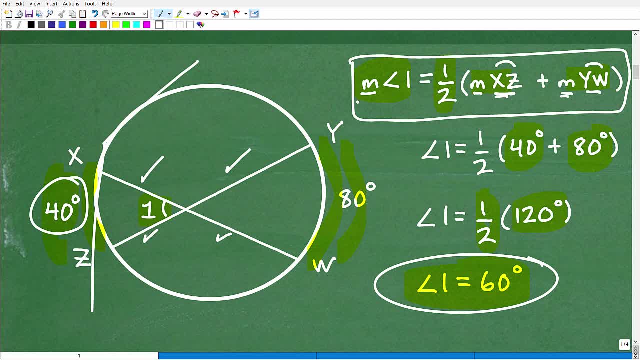 They're not difficult. But again, once you're dealing with a lot of formulas, they're easy to confuse, And the only way you're going to get good at this is to really be able to recognize the situation, use the right formula, and then you're going to be able to do the problem. 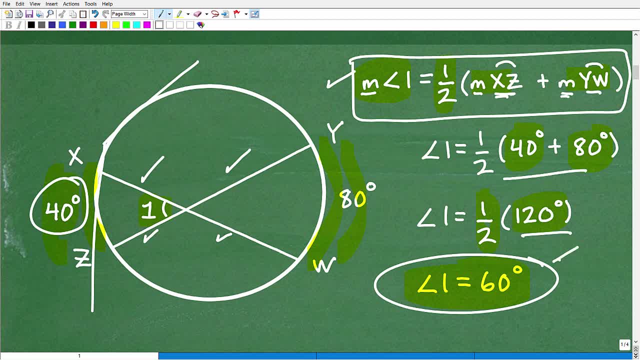 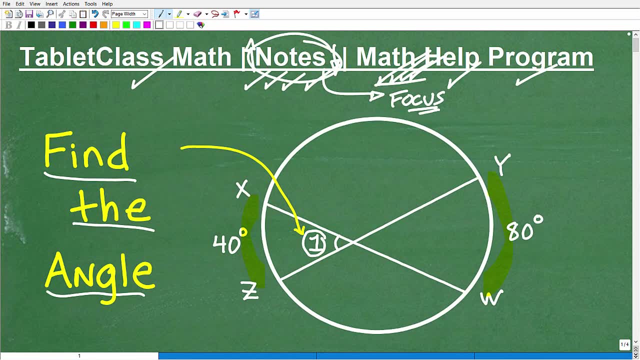 And then obviously do the simple calculations to get the right answer. Okay, So just a quick video on circles. Circles is a huge topic. by the way, on a lot of tests They come up pretty frequently. Let's say, if you're taking the SAT or ACT, I wouldn't be surprised if you do see. 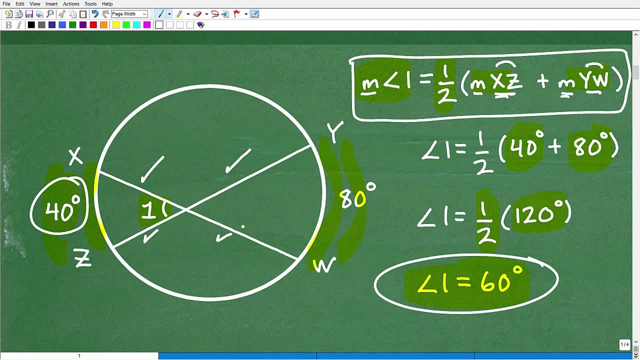 of these formulas. So we're going to go ahead and plug in the information, So we're going to particular lengths here with these chords. There's other things we can be doing, There can be other situations with tangents and things along those lines. So again, it's not just one. 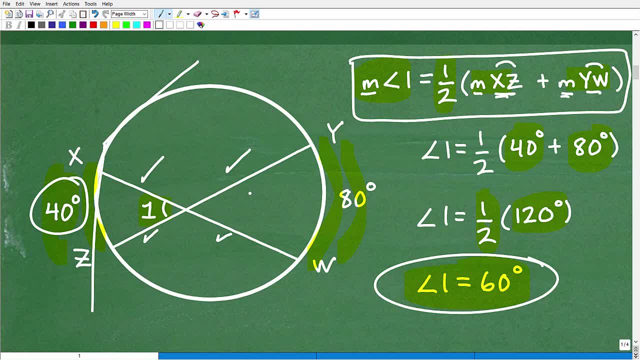 formula you need to know, especially with respect to circles in geometry. There's quite a bit of formulas. They're not difficult, But again, once you're dealing with a lot of formulas, they're easy to confuse And the only way you're going to get good at this is to really be able. 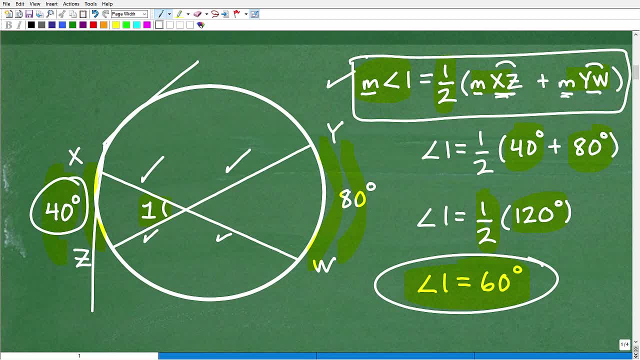 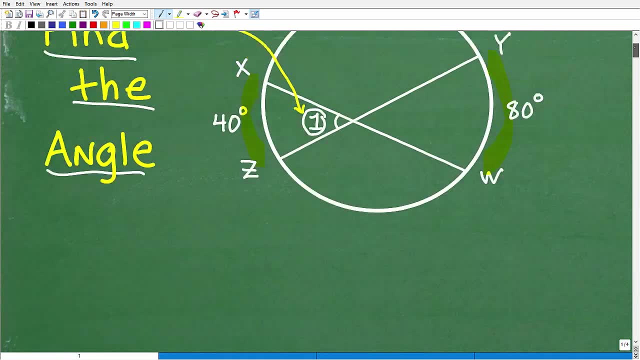 to recognize the situation, use the right formula and then you're going to be able to do the formula and then, obviously, do the simple calculations to get the right answer. Okay, so just a quick video on circles. Circles is a huge topic, by the way. on a lot of tests They 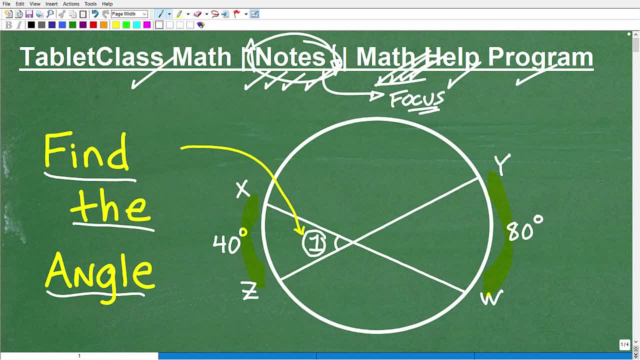 come up pretty frequently. Let's say, if you're taking the SAT or ACT, I wouldn't be surprised if you do see some questions on circles. So you know this is a generally speaking. in most geometry courses this is like a complete, full chapter: everything you learn about circles. So 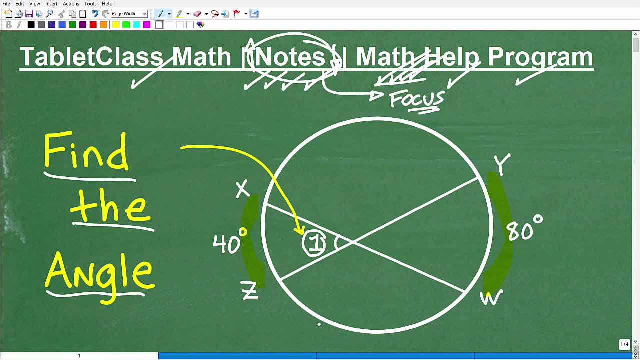 it's a bit of material and knowing how to do problems like this is, for sure, one of the things that you will be facing. So hopefully this little video helps you out on this particular type of problem. But again, watching this video is not enough. You have to practice this material and 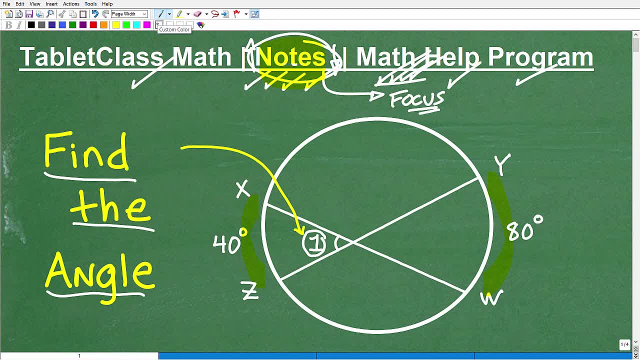 make sure all this information is in your notes, Okay, so if this video helps you out in some little tiny way, or maybe a big way, please consider smashing that like button, And if you're new to my YouTube channel, please consider subscribing. I've been on YouTube for 10,. 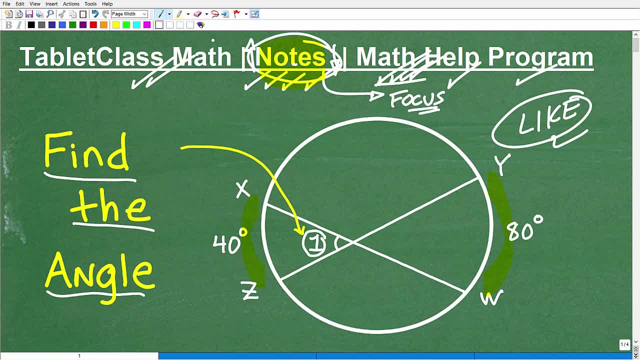 plus years. So I already have tons of videos on my channel organized from basic to advanced. If you go onto my- my YouTube channel you'll find a geometry playlist. So a lot of my geometry videos which I've done, quite a few on different topics- you can find there. But my best math help will. 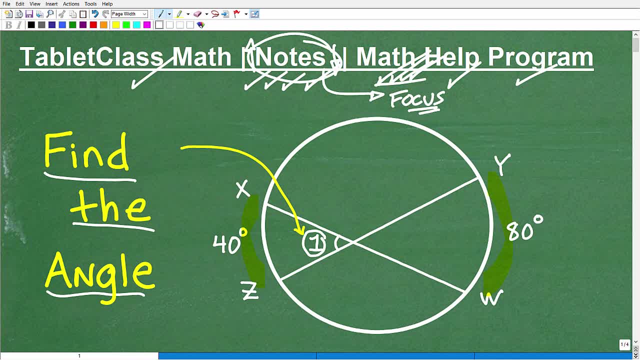 some questions on circles. So you know this is a generally speaking. in most geometry courses this is like a complete full chapter: everything you learn about circles. So it's quite quite a bit of material, And knowing how to do problems like this is, for sure, one of 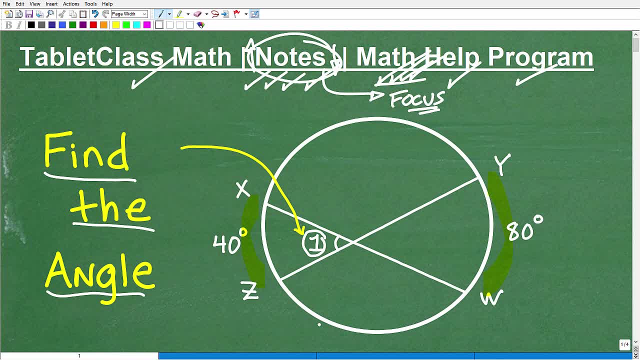 the things that you will be facing. So hopefully this little video helps you out on this particular type of problem. But again, watching this video is not enough. You have to practice this material and make sure all this information is in your notes. Okay, So if this video helps, 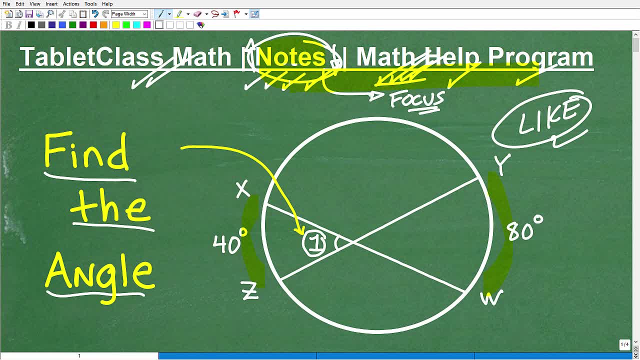 definitely be within my math help program, And if you are needing help in high school level geometry or just in geometry in general, you'll want to check out my geometry course. it could help you out. Okay, so, with that being said, I definitely wish you all the best in your